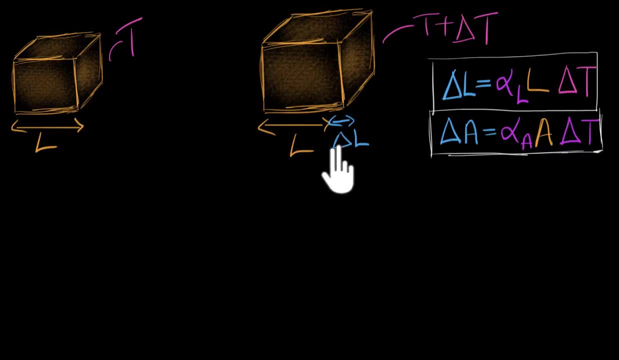 Temperature increases by delta T, The length on all sides increase by delta L And we need to calculate what is the change in the volume. Again, we know how to calculate changes in length, So we need to connect volume and length. Now is the great time to pause the video. 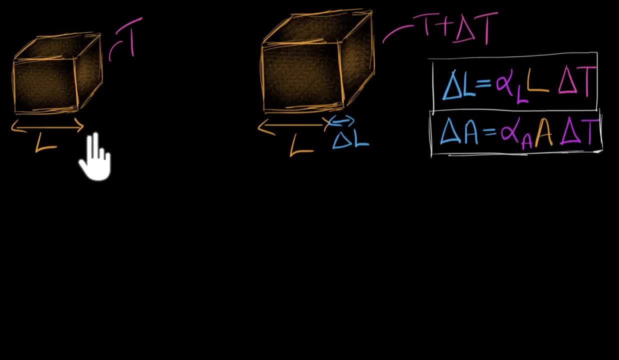 and try to derive this yourself. The steps are very similar to how we derived the expression for the change in area in a previous video. So if you need some refresher or you're required to just revise it, go back, watch that video, come back over here. 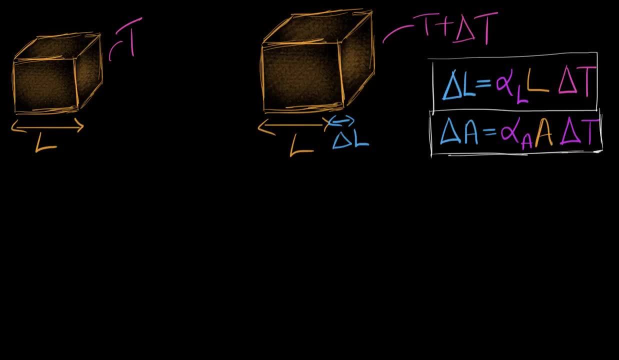 take the challenge. All right, let's do it. What is the connection between volume and length? How do you calculate volume of a cube If you know that volume of a cube V is just L cubed, So this would be the initial volume. 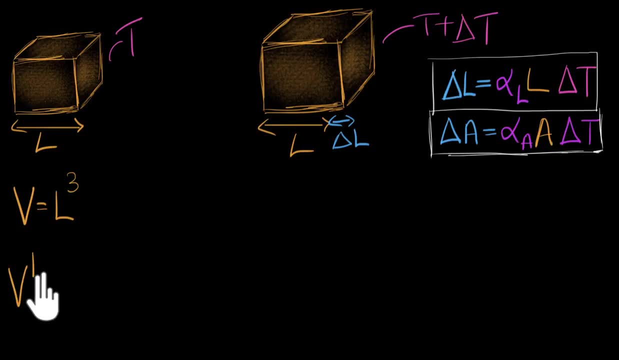 What would be the final volume? Let's calculate that over here. Final volume: V dash. well, that would be the new length cubed. The new length is L plus plus delta L, the whole cubed. So the change in the volume, delta V. 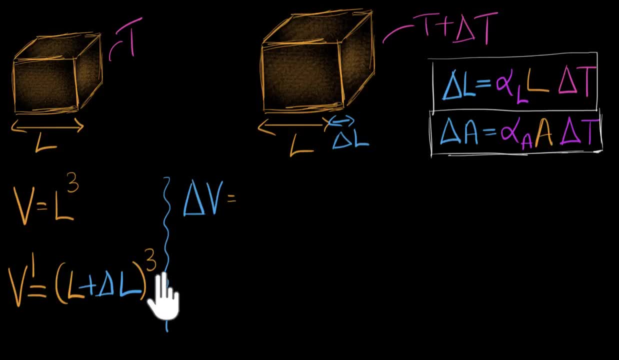 that's going to be the final volume, which is this number, L plus delta, L, the whole cubed minus. L cubed minus initial volume, L cubed: Well, more algebra. So just cube this whole thing, All right. so we need to remember. 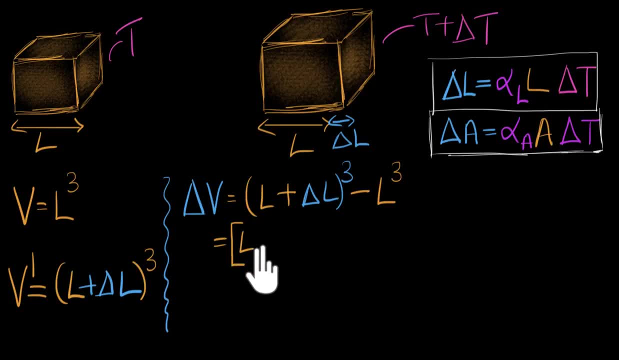 what is A plus B whole cube? formula A plus B whole cube is A cubed plus B cubed, B cubed plus three A B, three A squared B, three A squared B plus three B squared A. 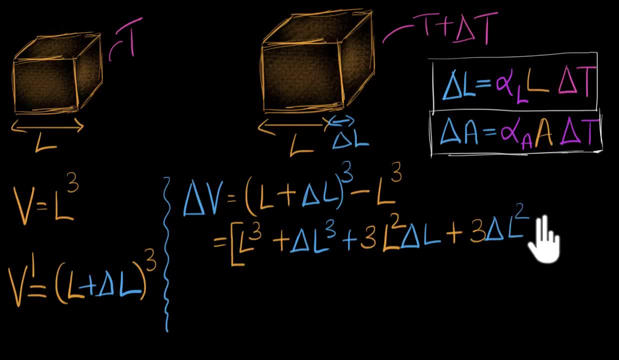 three: B squared A. Okay, you can pause over here and just check if everything is fine And notice L cubed cancels. So that's equal to well, we can do the same thing, what we did earlier: A, delta, L cubed and delta L squared L. 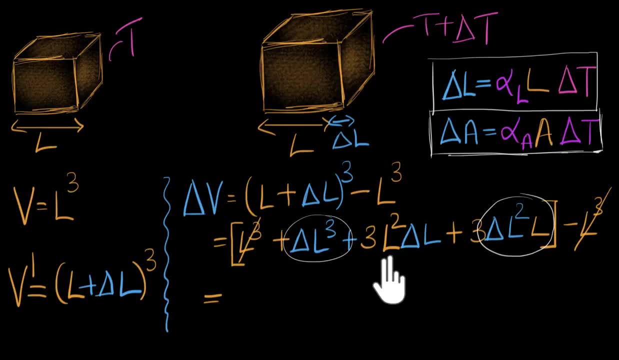 The whole thing. these two things can be neglected because they are very tiny compared to this number: L squared times delta L. Take the same example that we did before. Convince yourself, Do that yourself. You will see that you can totally neglect them. 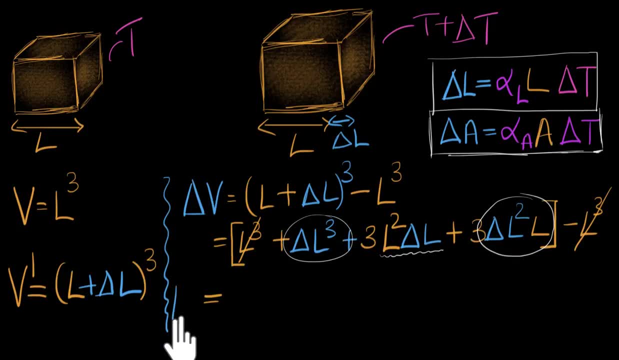 provided delta L is very small, And so we now end up with, let's see delta V equal to three times L squared times delta L. What is delta L? Ooh, we know that That is alpha L. That's over here. 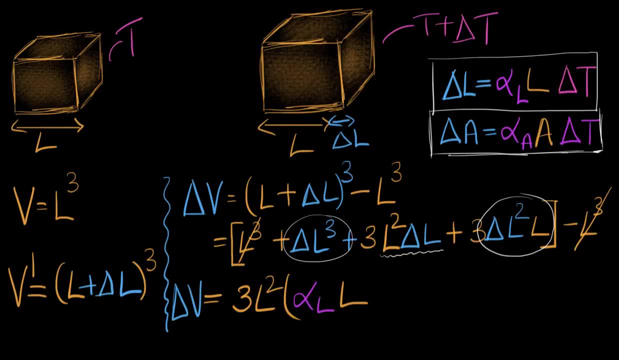 Very similar to what we did before: Alpha L times L times delta T, times delta T. And so that gives us- let's see one last step. You have three alpha L, three alpha L times L cubed. L cubed is the initial volume. 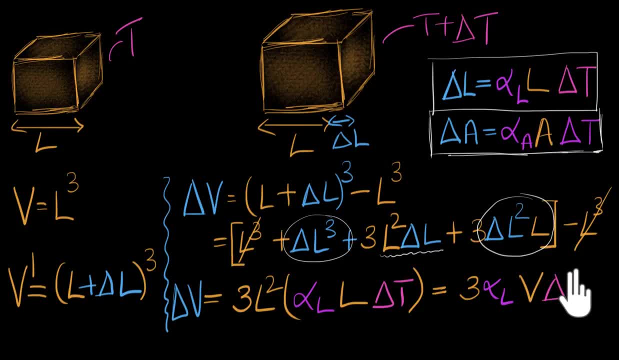 initial volume times delta T times delta T. And let's box this. Okay, I'm just gonna box this one And see what we get. now We get a very similar expression, like we did before. Delta V equals some number times original volume times delta T. 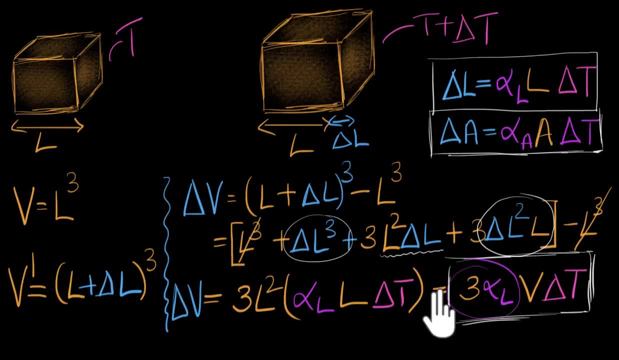 So any guesses? what do we call this number? as If you guessed, we will call this as alpha V: volume expansion coefficient. And you're absolutely right: Volume expansion coefficient, Volume expansion coefficient. And so notice, alpha V is going to help us. 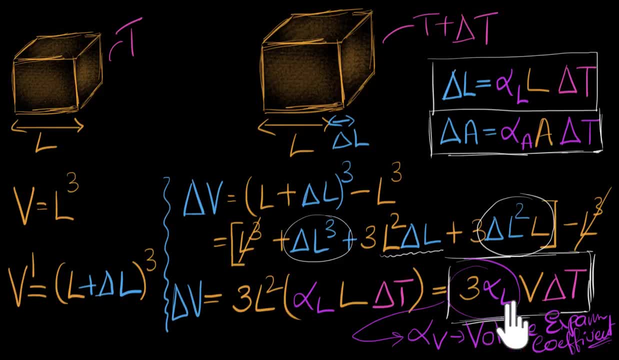 calculate changes in volume, And alpha V is three times alpha L, Just like how alpha A is two times alpha L. Now you may wonder that we derive these expressions for delta A and delta V for very simple shapes like squares and cubes. But do they work in general? 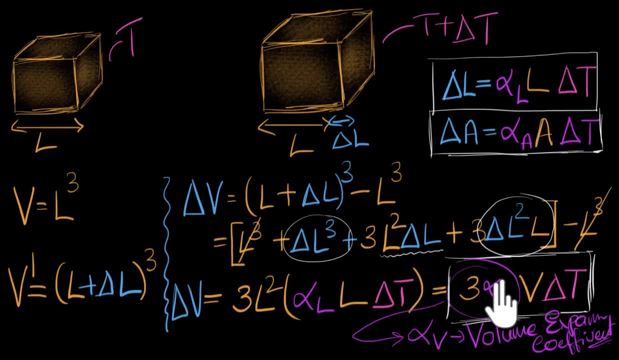 The answer is yes, they do, And it would be a great exercise to try and derive it for some other shapes, like, say, a rectangle, or maybe a circle, or maybe a sphere or a cylinder, and see that you get exactly the same result. But whatever the shape may be, 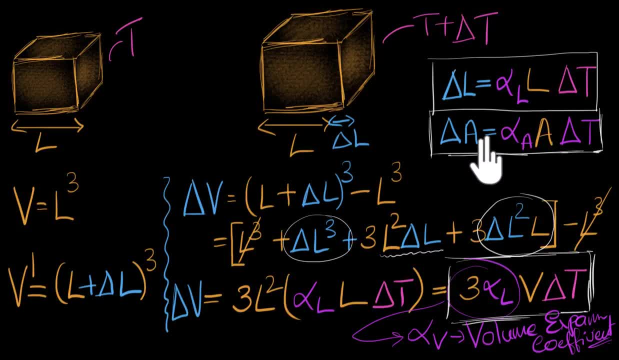 as long as the expansions are small enough, we will see that these expressions hold true. One last thing we'll do is quickly take a look at a table which has the values of alpha L and alpha V for some materials. So here it is. 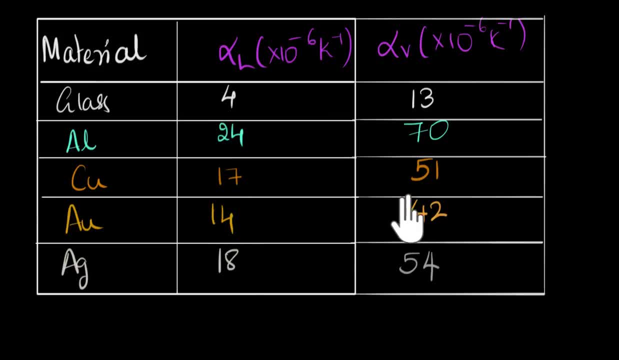 Take a look at the values of alpha V and alpha L of different materials and you can pretty much see pretty much: alpha V is three times alpha L. So you can see that alpha V is three times alpha L. So you can see that alpha V is three times alpha L.